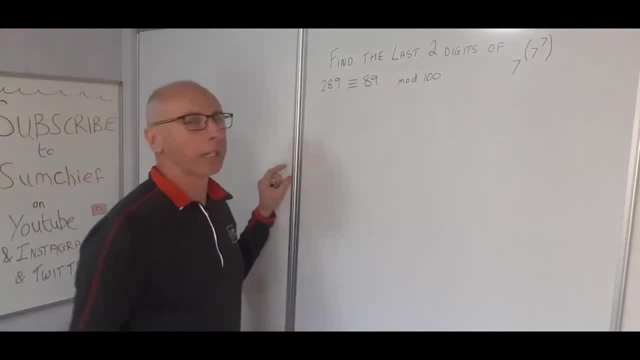 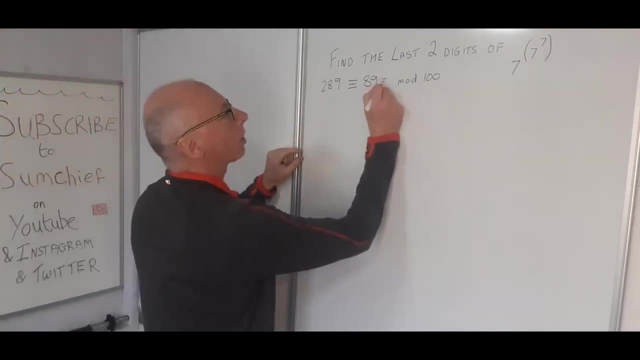 two digits. Now this number here we need to between 0 and 99 to give us our correct congruence, because this is also congruent to minus 11 mod 100.. Obviously, the minus 11 is not what we want. We want the positive. 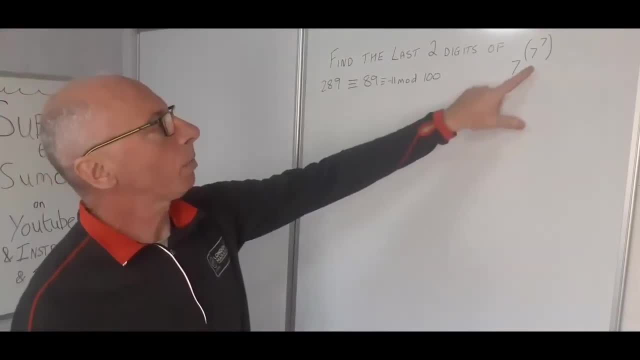 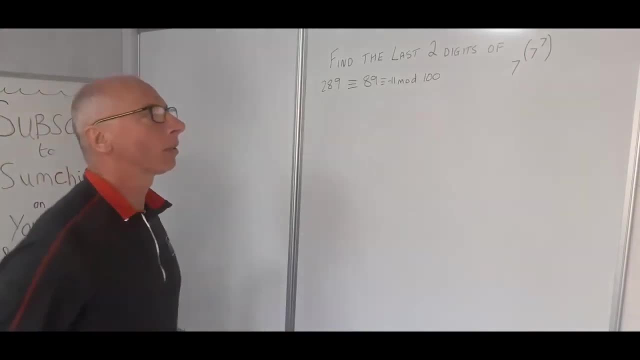 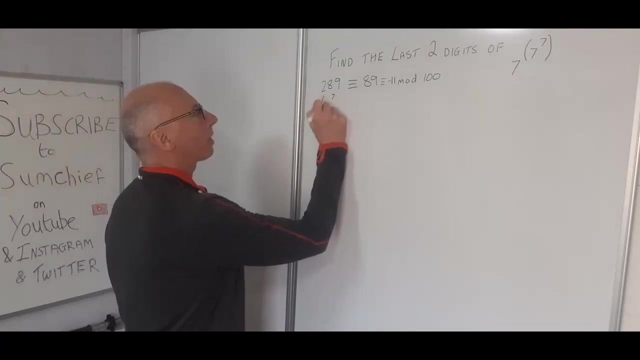 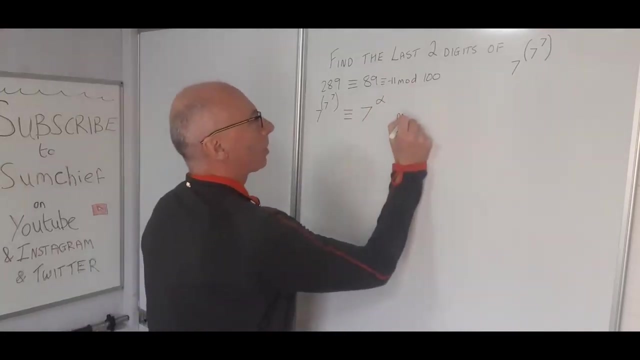 Okay, now the first place to start would be for Euler's phi function. We need to plug in some value for this using Euler's phi function. So ideally, what we're looking for is 7 to the power of 7 to the power of 7 is congruent to 7 to the power of some number. alpha mod 100. 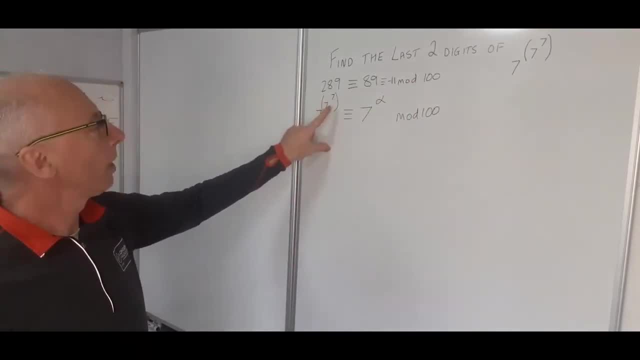 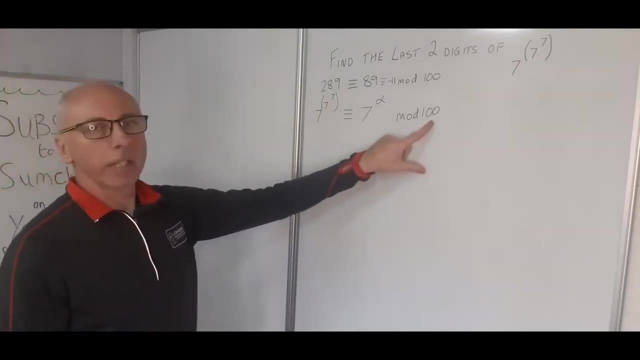 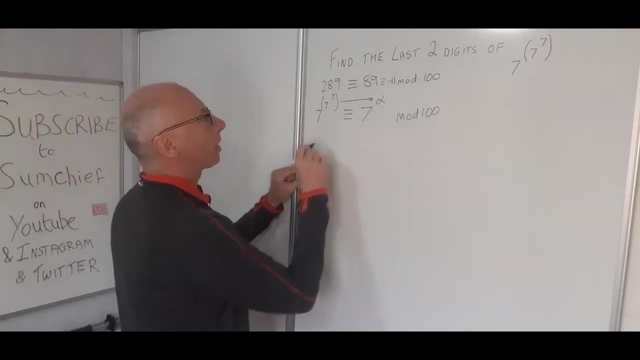 If we find what 7 to the power of 7 is congruent with 100, that's not necessarily going to work for this question here. So what we're looking for is this bit. here is what we're looking for now, to get to this bit. So what we want is 7 to the power. 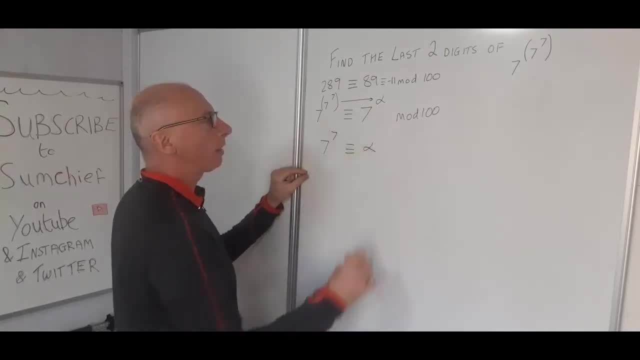 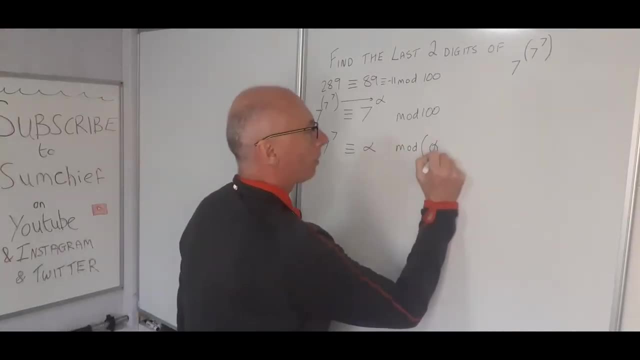 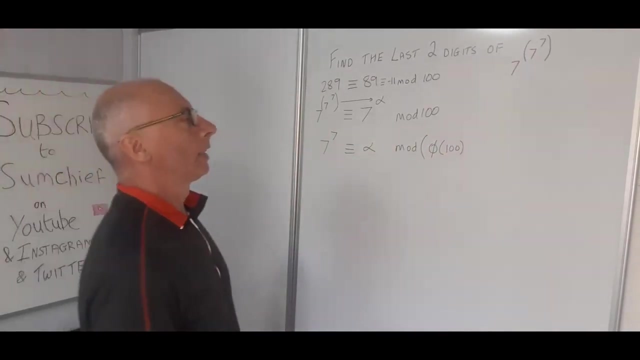 of 7 is congruent to alpha modulo. Now, instead of writing the 100, I'm going to write phi of 100.. I'm going to leave the bracket open for one minute Now for a 5100. we can work this out. It's a. 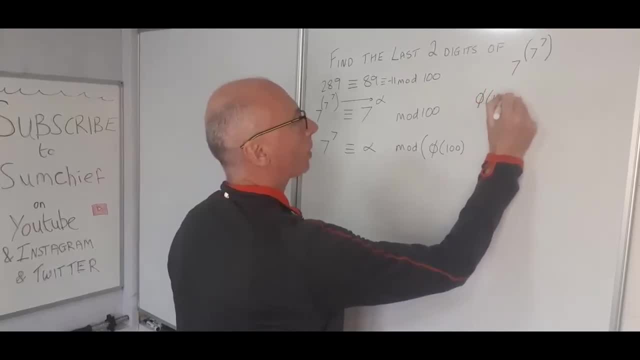 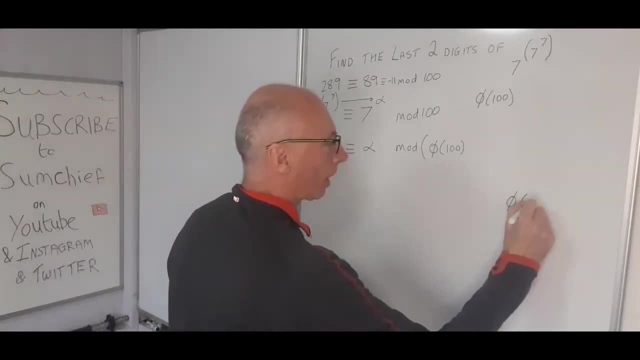 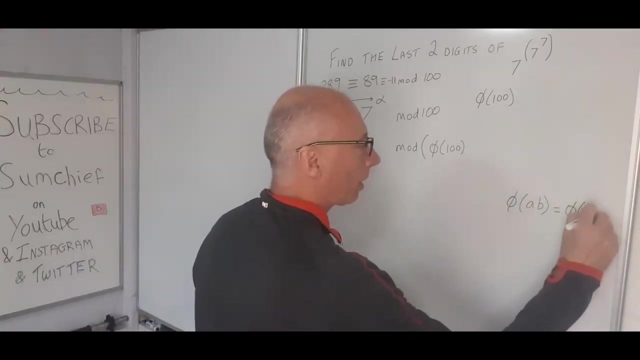 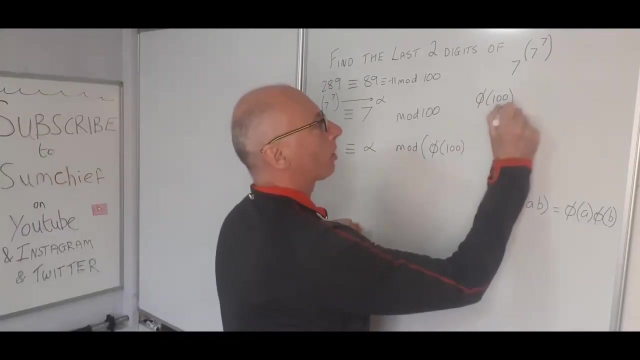 multiplicative property 6 of 5100.. Okay now, using the formula. using the formula here, phi of a, b. so a times b is equal to 8 of 5B but 100. we can break this down into phi of 25 and phi of 4.. 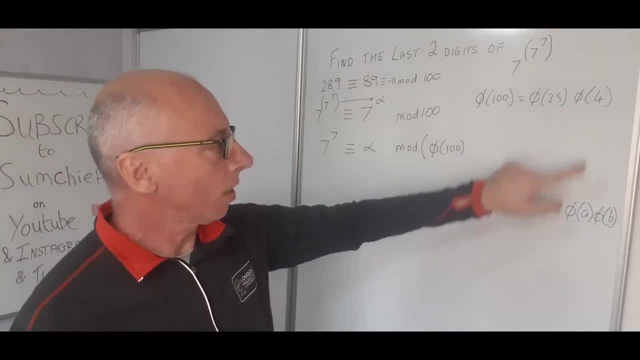 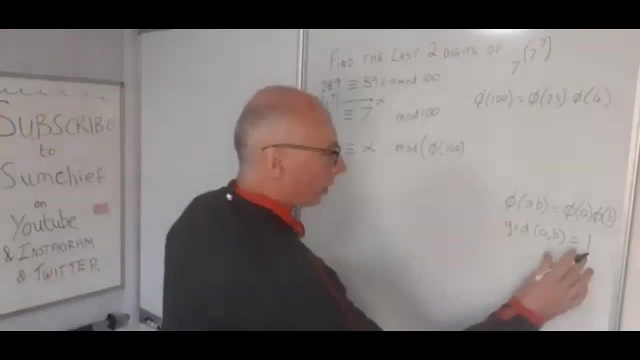 But this gives us a bit of a problem, because this is only valid if the gcd of a comma b equals 1.. So gcd of a and b is 1. that is correct. but we also need a and b to be prime numbers, which is not the case, So we've got a situation here. 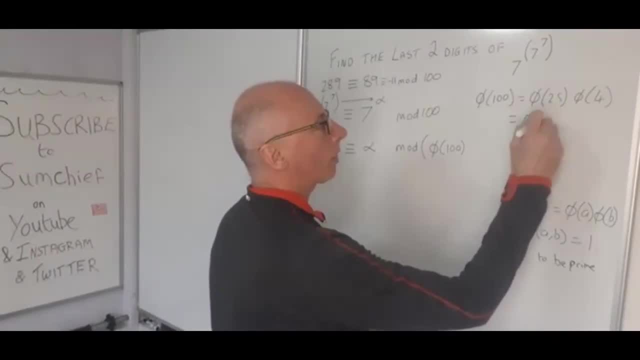 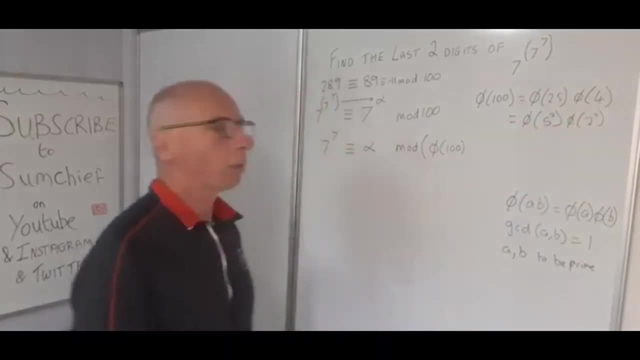 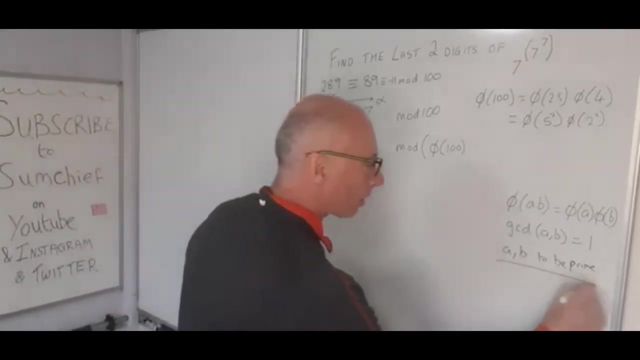 where we've got phi of 25, we know is 5 squared and phi of 4 is 2 squared. Now there's a formula we can use for that. so just put this in a box. now we can say phi of a prime number to some power. let's call it a. this is the same as 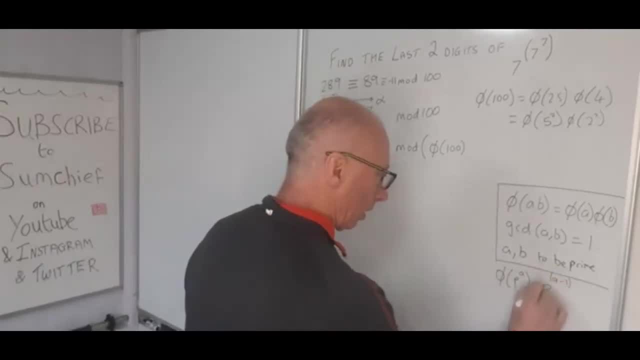 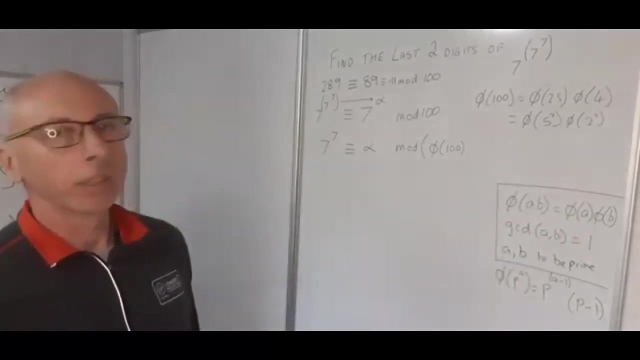 p to the a minus 1, so that's all in the power of that prime number, which is just the 1, and then we multiply that by the prime number minus 1.. So this we can use because 5 and 2 are both prime numbers. So let's work these out separately. 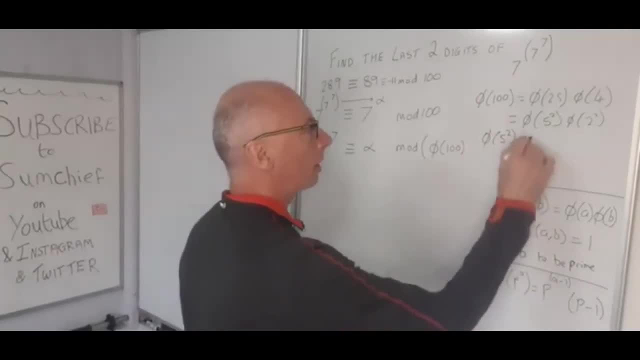 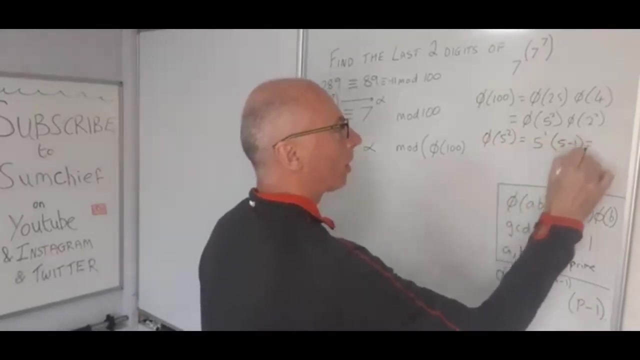 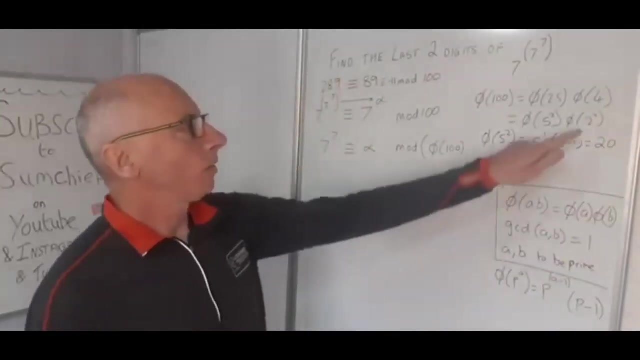 So phi of 5 squared using this formula, that's going to be p, which is 5.. And then we multiply that by the prime number minus 1.. So 5 minus 1.. So that's going to be 5 times 4, which gives us 20.. And then likewise with the phi of 2 squared. 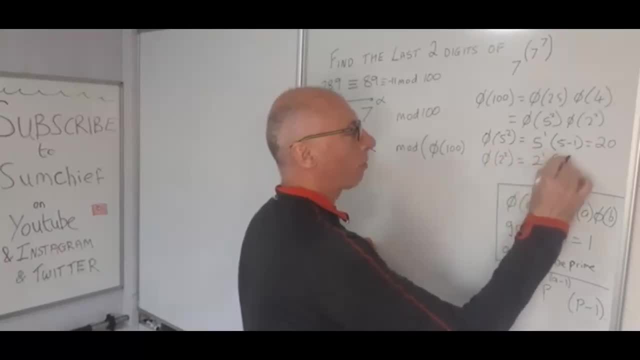 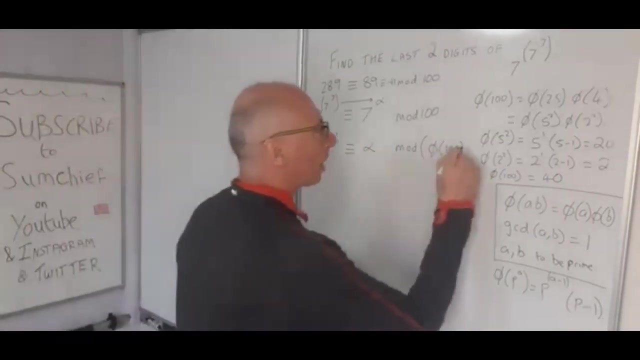 So then it's going to give us 2 to the power of 1 times 2 minus 1.. So 2 times 1 is 2.. So therefore, phi of 100.. So therefore, phi of 100 equals 40. So I'm going to write in here: equals 40. Just squeeze that there for our modulus. 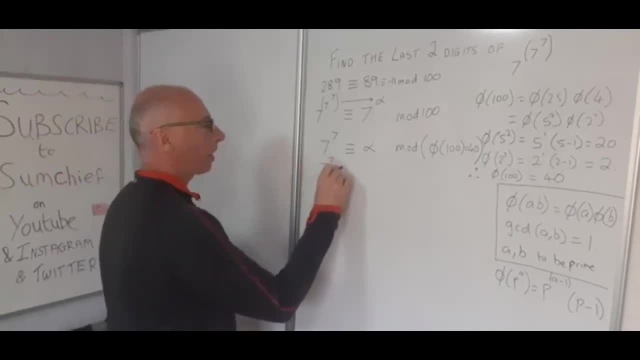 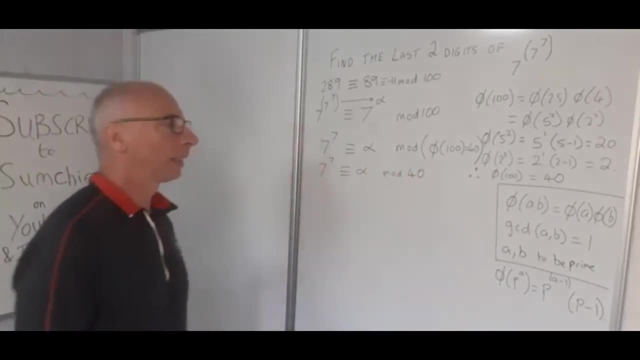 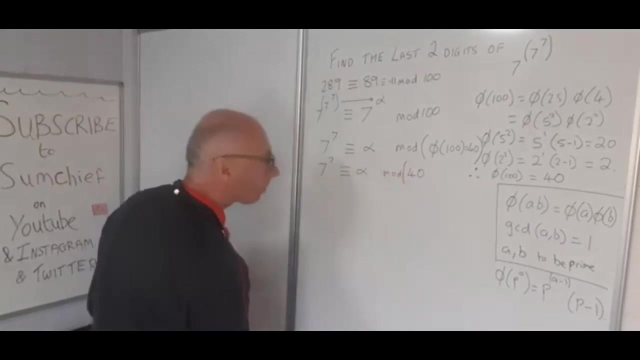 Okay, so now, starting on a new line, 7 to the power of 7 is congruent to some number, alpha modulo 40.. Okay, now 40 is still a big number, So I'm going to go one more level on this one. So now I'm going to change this to phi of 40 and then calculate what phi of 40 is. 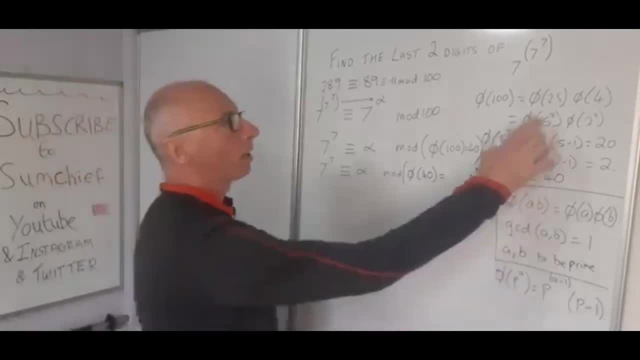 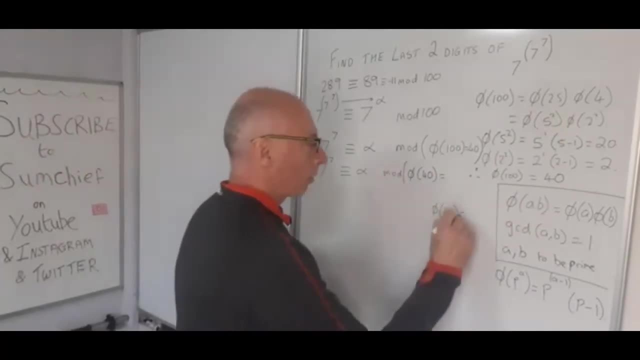 Okay, so now it's going to do this working out on here the way we did this. So phi of 40. Now that's going to be equal to phi of 8 times 5.. So phi of 8 is 2 cubed And then phi of 5.. 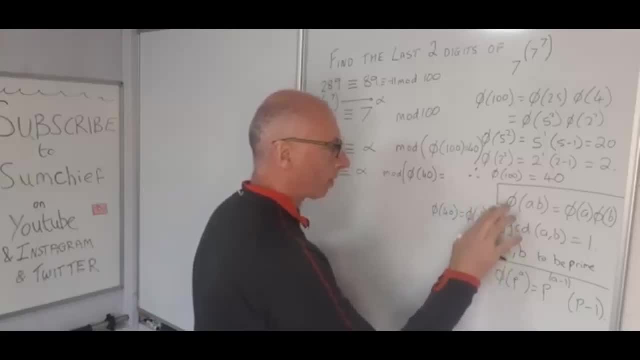 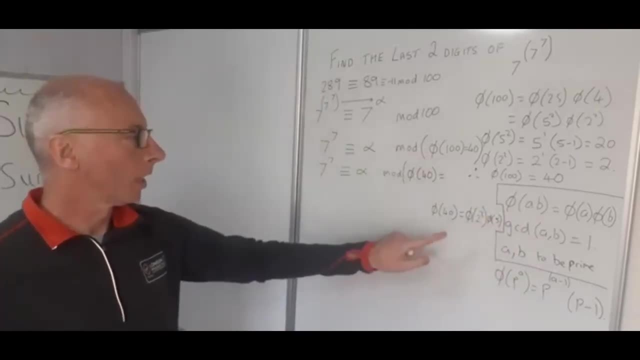 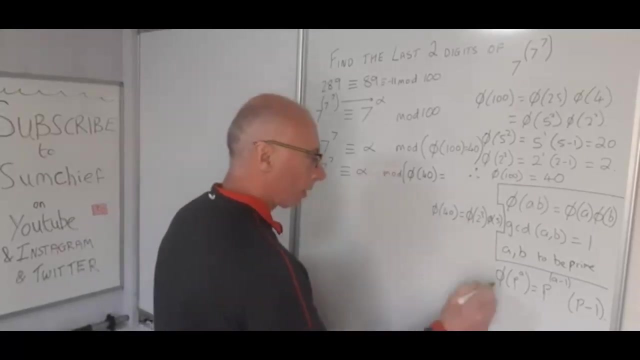 Let's just give it a little bit of space in the box. Phi of 5.. Now, phi of 5 is okay, That's the prime number. But phi of 40. Let's see. Let's see, see what we got for, sorry. phi of 2 cubed. So phi of 2 cubed. that equals p to the a minus 1 times p. 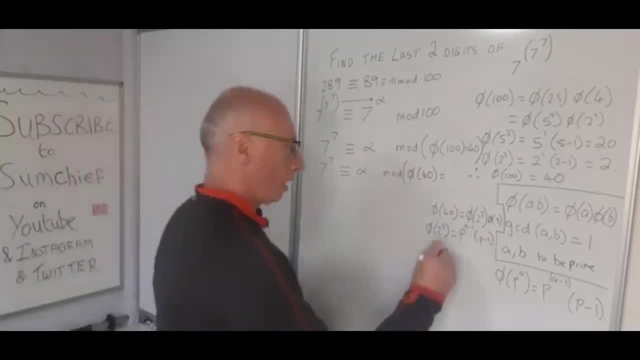 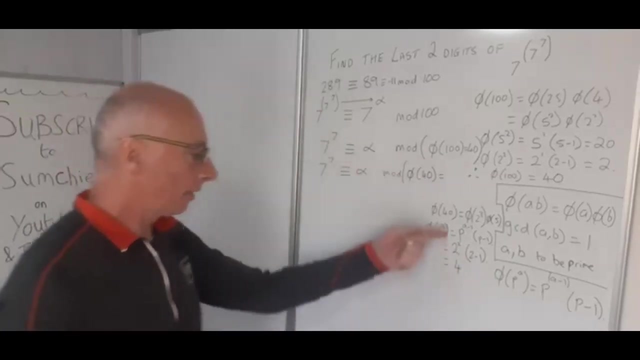 minus 1.. That's our formula, p is our prime, so that's 2.. 3 minus 1 gives us another 2.. Then the prime minus 1 is just 2 minus 1.. So 2 squared is just 4.. And then phi of 5 and the answer to that. 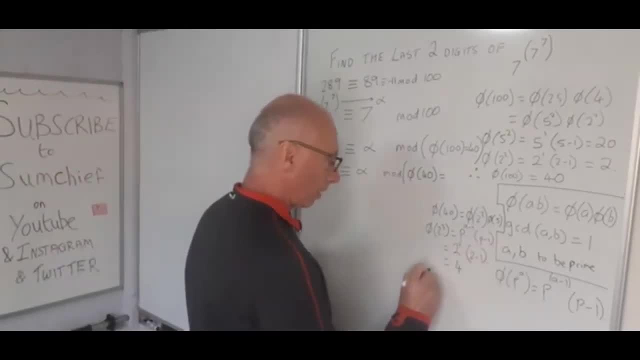 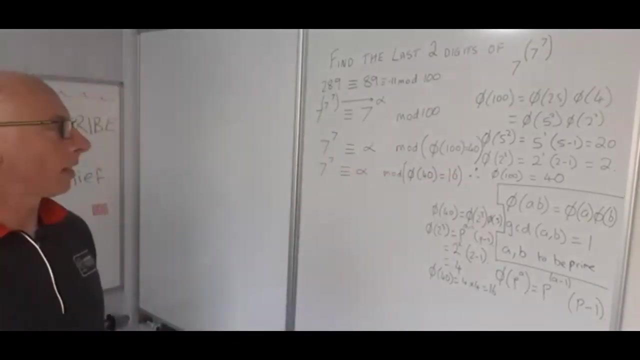 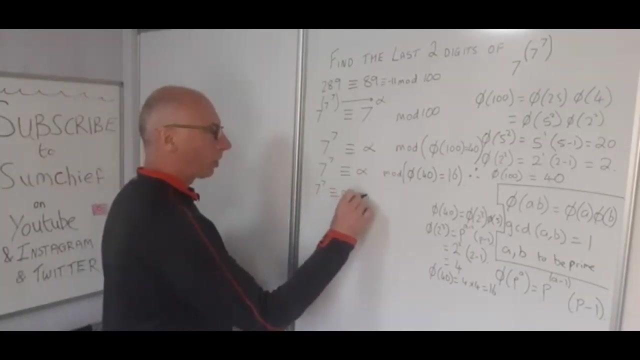 is 4.. So therefore, phi of 40 equals 4 times 4, which equals 16.. So 16. when you're working with the number 7, that's going to make things a lot easier. So 7 to the 7 is congruent to alpha modulo 16.. 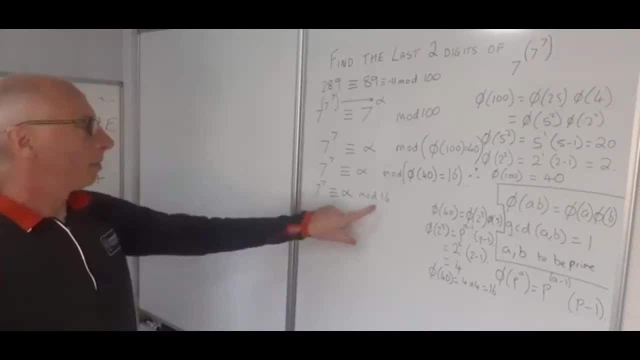 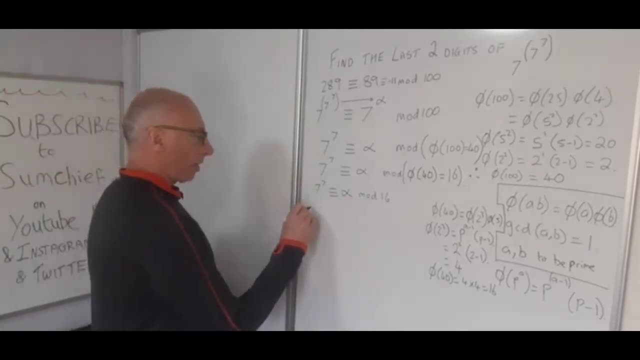 Okay, so we can work with that 7 modulo 16.. We can use some powers of 7 and stuff like that. So 7 to the 7 is 7 squared times 7 squared times 7 squared times 7.. Let's put: 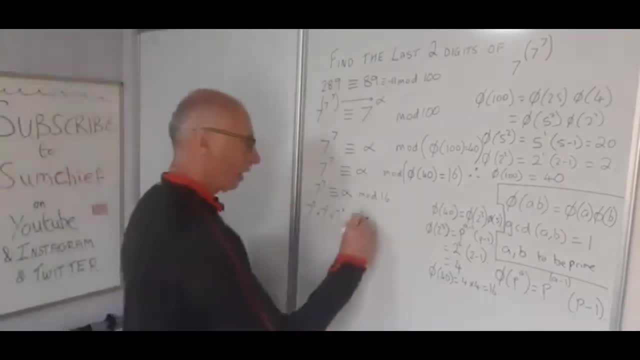 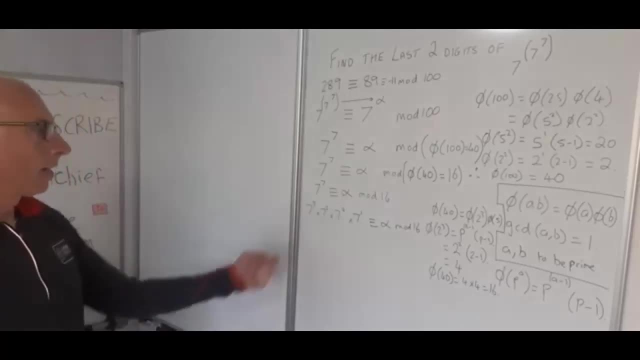 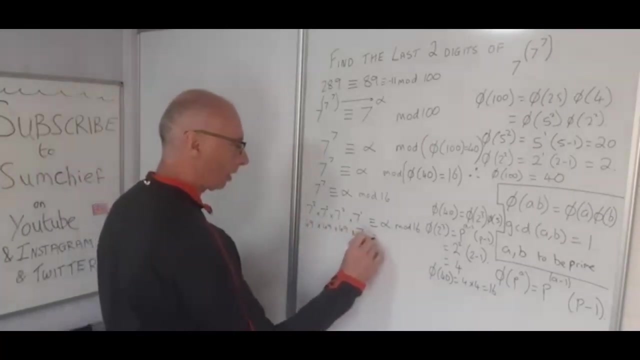 number 1 there. So that's our 7 to the 7.. That's congruent to the number alpha mod 16.. Okay, 7 squared is 49. So we've got 49 times 49 times 49 times 7, congruent to alpha mod 16.. 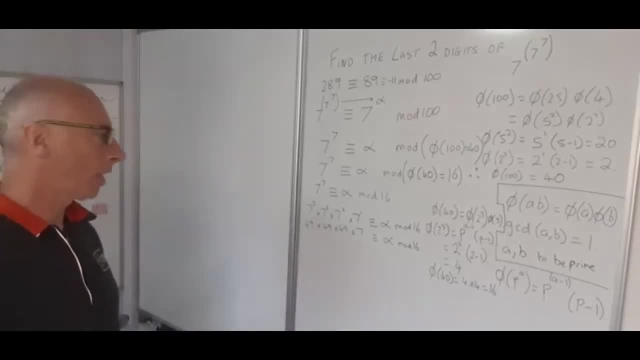 Now you can plug that in your calculator and see what you get, but that's going to be pretty hard going. Well, it's a nice little shortcut, Because 49 is congruent to 1 mod 16. So we just plug in a 1 for the 49's. 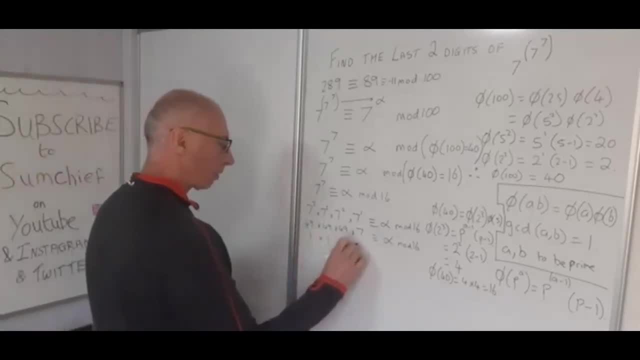 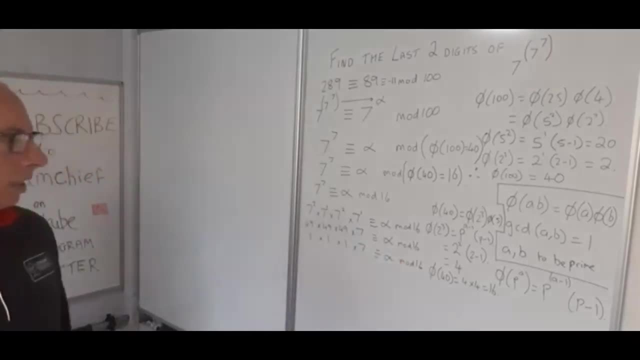 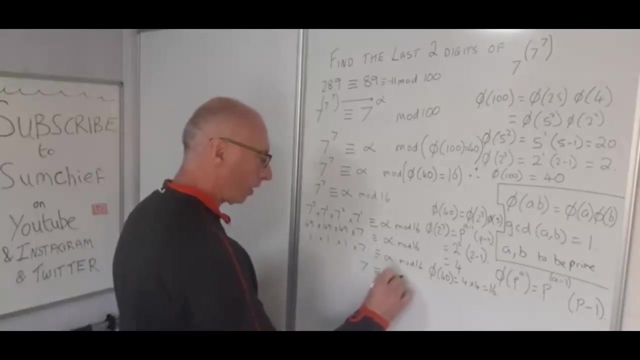 So now we're left with 1 times 1 times 1 times 7 is congruent to alpha mod 16.. So now we've got 1 times 1 times 1 times 7.. That's all good. 7 is congruent to alpha mod 16.. So therefore, we let our alpha equal 7 to 1.. 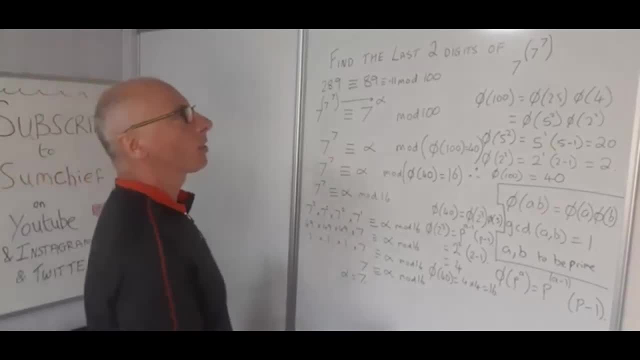 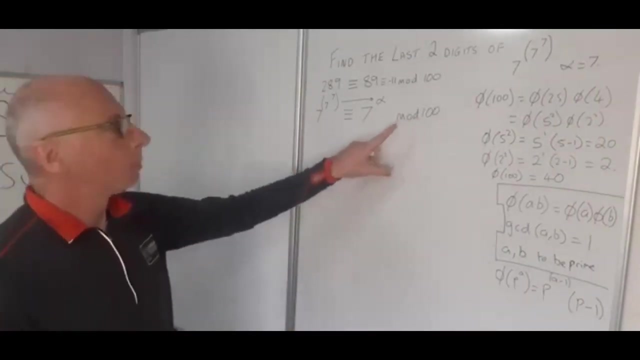 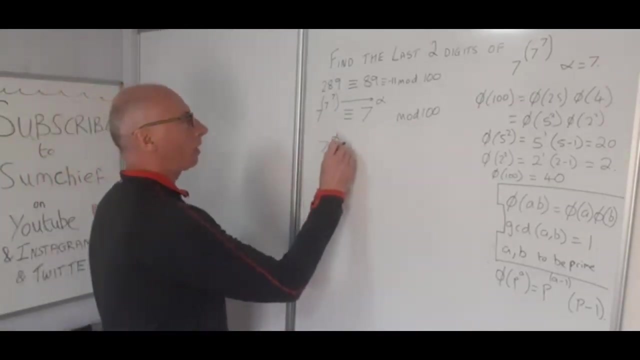 7.. So let's just write this up here: alpha equals 7.. So now I'm going to take this off the board and resume it at this line here. So now my question is: we need to go back to modulo 100 to find our answer. So we need 7 to the alpha is congruent to our 7.. Well, alpha is 7,. 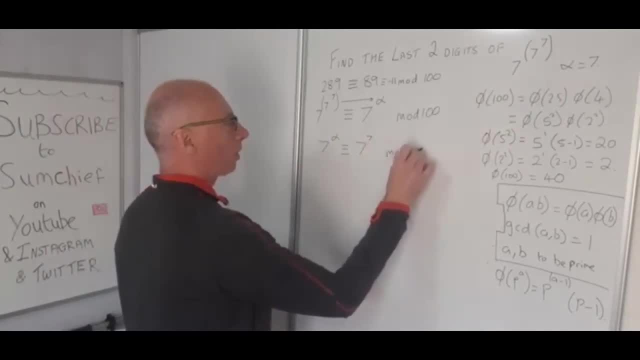 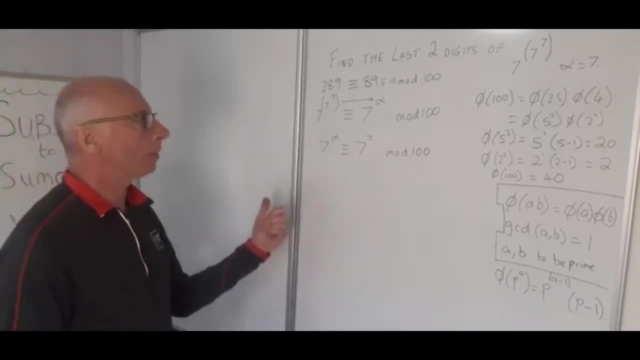 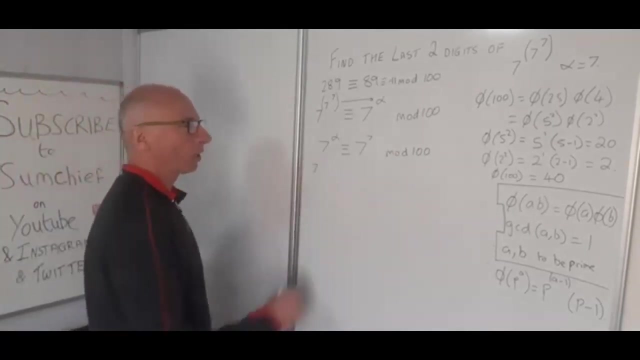 7, mod 100.. Okay now, what can we do with this 7? We need some powers of 7 to help us with our mod 100.. Now, the 7 squared is not going to work because that's 49. But we know that 7 cubed. 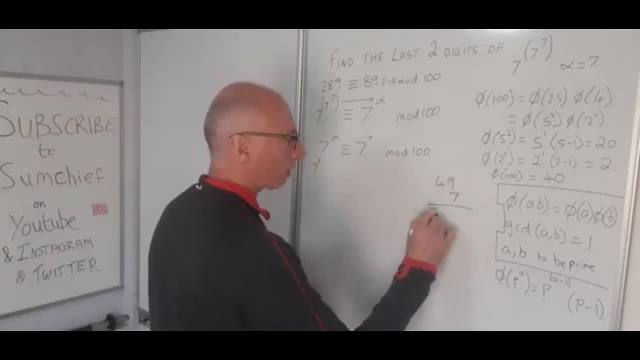 49 times 7.. 7- 4's are 28, so that's 280.. 7- 9's are 63.. So that's that one. So that's 3 4 3, which is congruent to 43 mod 100.. Just put an m there for. 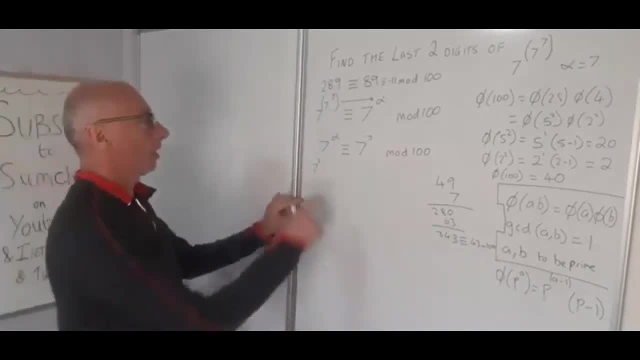 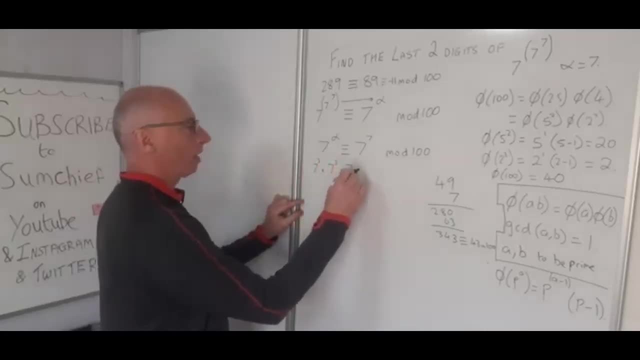 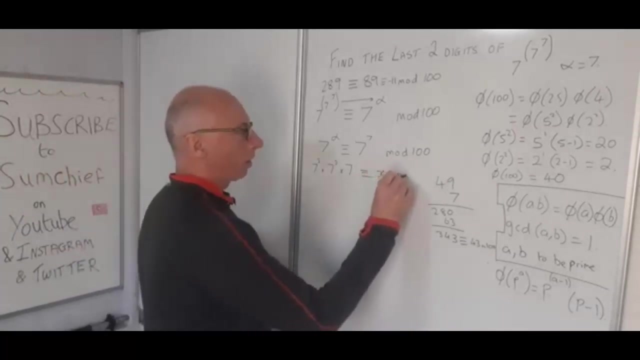 short, Just a quick calculation. So that's 43.. So we can rewrite this: 7 to the 3 times 7 to the 3 times 7 is congruent with some number which I'm just going to call now. We'll call this x mod 100. 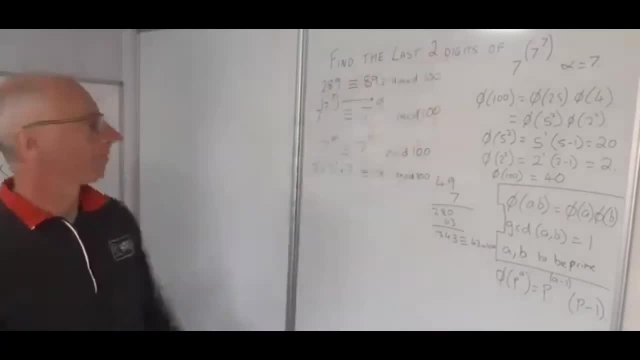 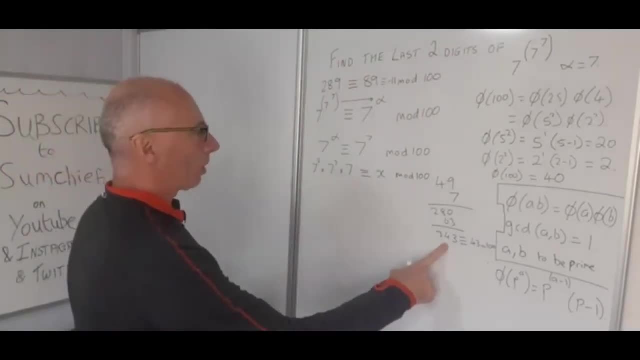 x will give us the answer to our question. So 7 cubed? Well, 7 cubed, we know, is 343 and mod 100 is just 43. So we substitute a 43 into these two and the 7.. So 43 times 43 times 7 is congruent with x mod 100.